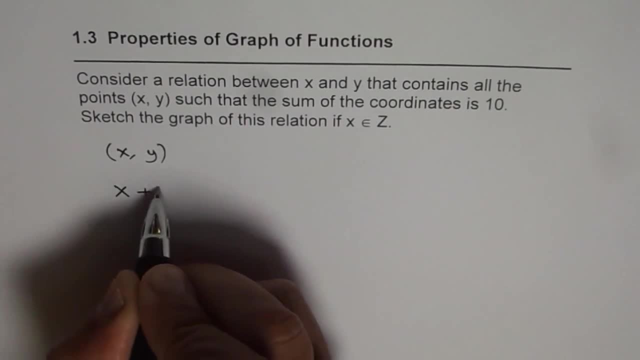 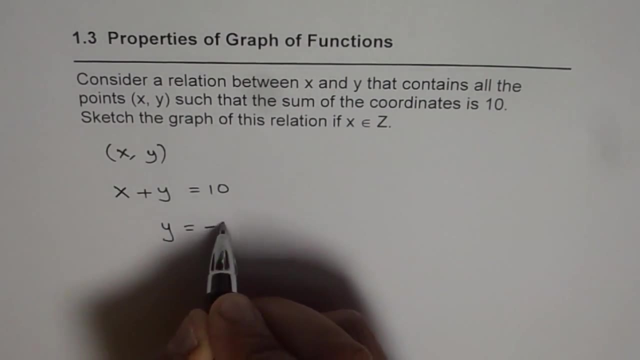 y are such that x plus y is equal to 10.. Now we can rearrange this equation and write: y equals to minus x plus 10.. So that is our function. f of x is equals to minus x plus 10.. And in this we are given a restriction that x belongs to integers. So we have to 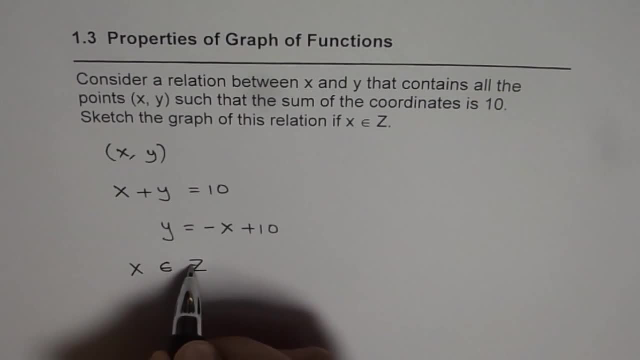 consider only integer values for x. 1.3. Properties of graph of functions. Consider a relation between x and y that contains all the points x and y that contains all integers. if x belongs to set of integers, So that is our function. So with that in mind, let us now sketch the graph. So that means there. 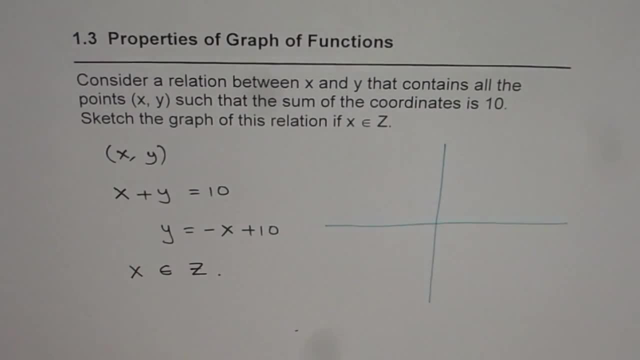 is our coordinate plane and we are looking for a few values first. We know it is a straight line. So if x is 0, in that case y will be plus 10, right, So y value will be- let us say, this is 10 for us, And if y is 0,, x will be plus 10.. Which is yourن and the magnitude? 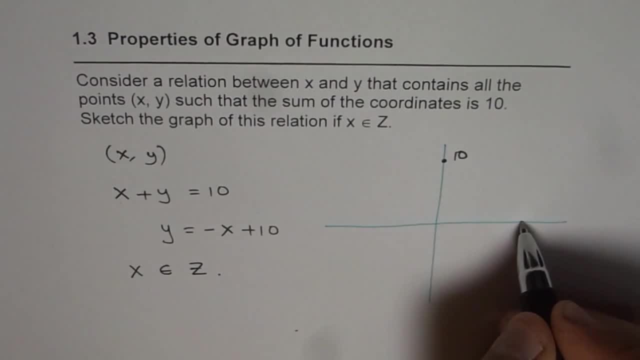 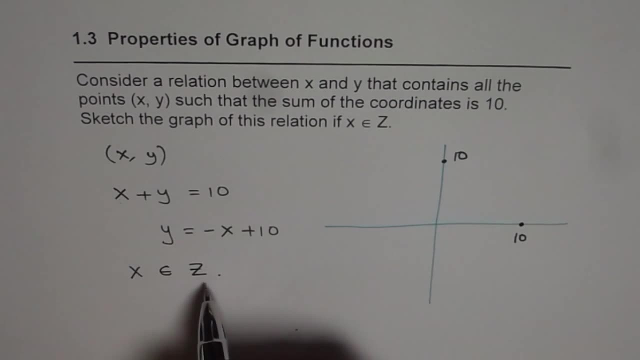 be plus 10. so let us say this is the x intercept 10 for us, and what we can have in between is any value of x. you can make table of values. so if x is 1, y is going to be 9. so if x is 1, y is going to. 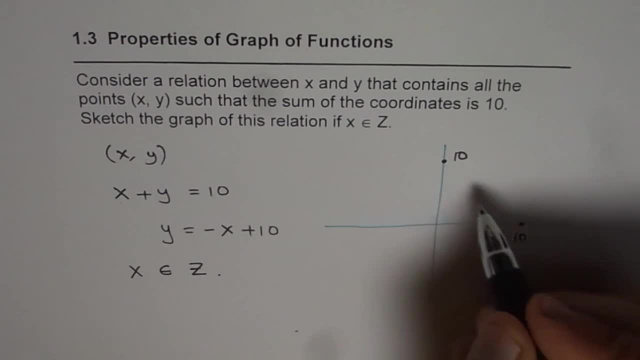 be 9. so likewise we'll have all the points which are kind of: so we can have 10 points like this. so x for x equals to 1, like this. so we'll have many points like this and it can be extended as shown here, right, so you can plot few points. so it is set of points which will add up to 10. 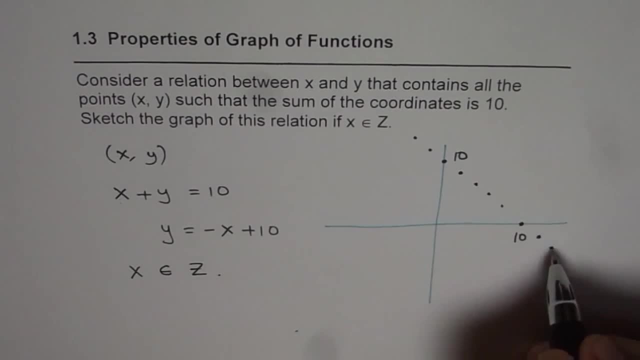 so that is how we are going to get the graph of it and this pattern is going to continue in both the directions. right, remember, you should not be joining them by a straight line, so put only the points there. so it's kind of a scatter plot with a straight line. so that is how. 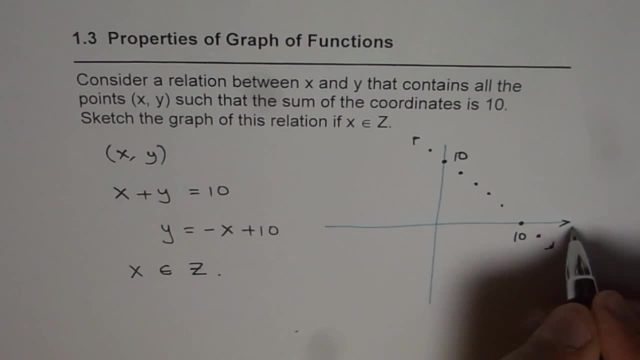 it will look like right. so that is your x-axis f of x on y-axis. that's the origin and that is how you are going to get the graph of this function. thank you.